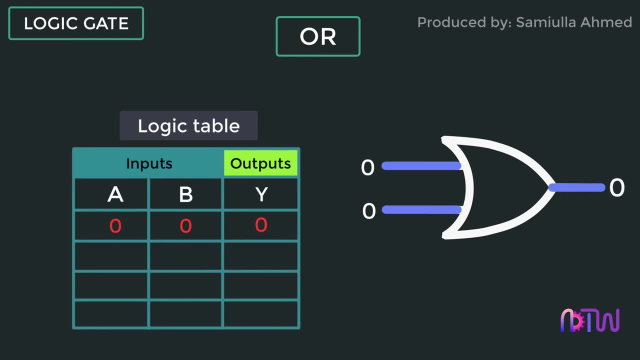 signal in A or B, the output will be 0, which indicates there is no signal in A or B. Now consider the second case. In this input A equals 1 and B equals 0. Since there is a signal in input A, the output will be equal to 1.. For our gate to give an output signal, there should be at: 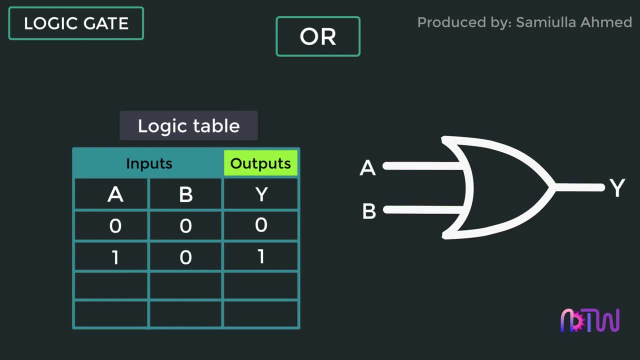 least one input signal. The third input signal will be: A is equal to 0 and B is equal to 1.. Since there is no signal in A or B, the output will be 0.. Since there is a signal in A or B, 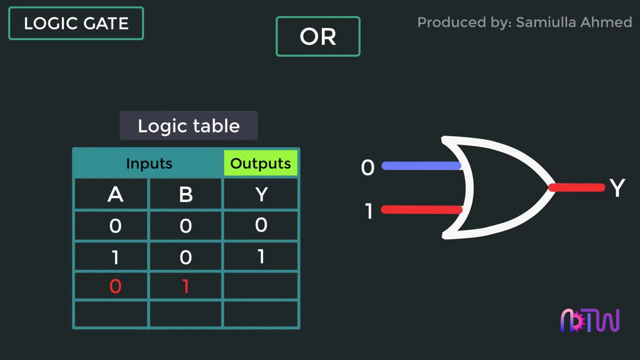 since there is a signal in one of the inputs. therefore, the output will be equal to 1.. And the final input signal will be: A is equal to 1 and B is equal to 1.. Therefore, output will be equal to 1, since there is an input signal in both A as well as B. 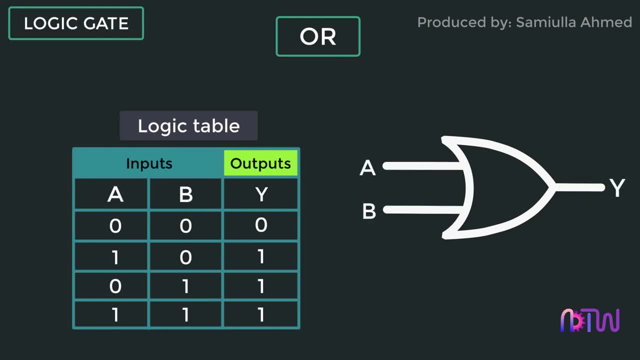 For the ease of remembering how our gate works, you can imagine it as a simple bulb with two switches. When switch A is on and switch B is off, the bulb will glow, Since it is getting the required supply If switch B is on and switch A is off. 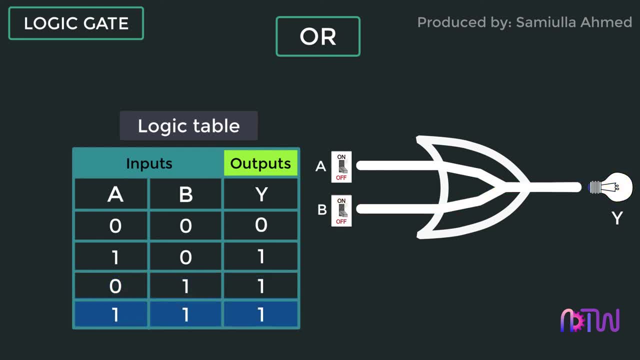 still, bulb will glow. And if both switches A and B are on, the bulb will glow. This is how our gate works. If you are enjoying this video, please give this video a thumbs up and if you are new to ADTW, Learn, click on the subscribe button. 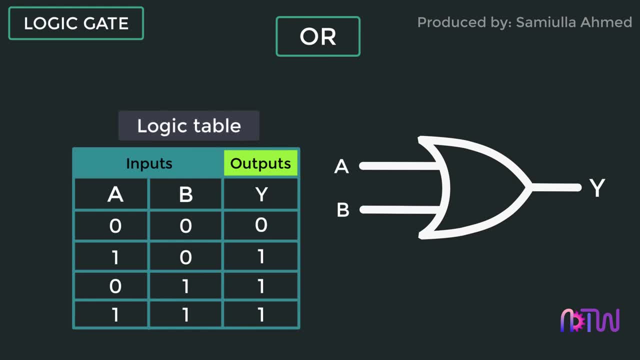 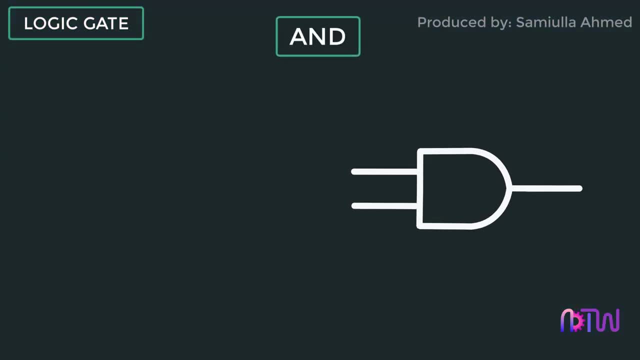 and turn on the notification to get new informative videos like this. Let's move on to next logic gate, which is AND gate. Similar to OR gate, AND gate also has two inputs, A and B, and one output, Y. The working of AND gate is based on the mathematical meaning of: 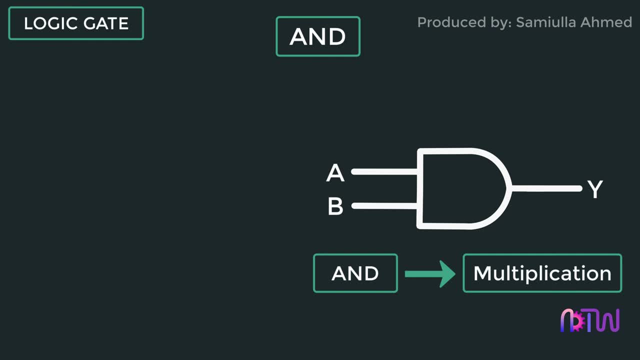 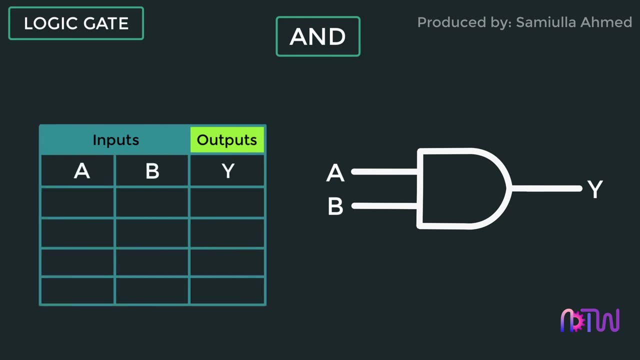 AND. that is multiplication. For the AND gate to give an output, both the input, A and B, should have a signal. Let's see the logic table for AND gate. It can have four combinations of input. The first input will be: A equals 0,. 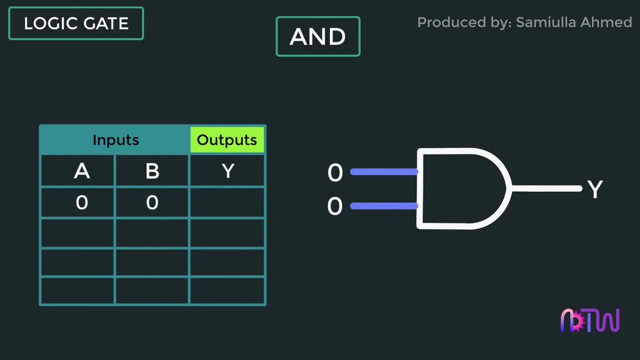 B equals 0.. Since both A and B have no signal, the output Y will be 0.. You can also get the output of AND gate by doing A into B. Since A equals 0 and B equals 0, 0 into 0 will give the 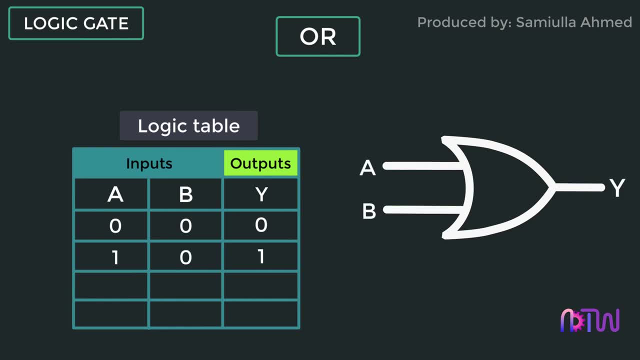 least one input signal. The third input signal will be: A is equal to 0 and B is equal to 1.. Since there is a signal in one of the inputs, therefore, the output will be equal to 1.. And the final input signal will be: A is equal to 1, and B is equal to 1.. Therefore, output will be: 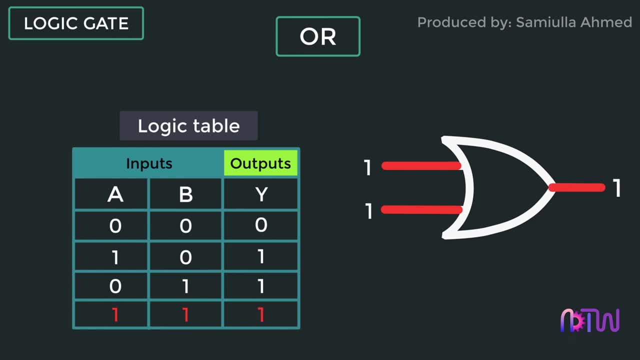 equal to 1,, since there is an input signal in both A as well as B. For the ease of remembering how OR gate works, you can imagine it as a simple bulb with two switches. When switch A is on and switch B is off, the bulb will glow, Since it is getting the required supply. 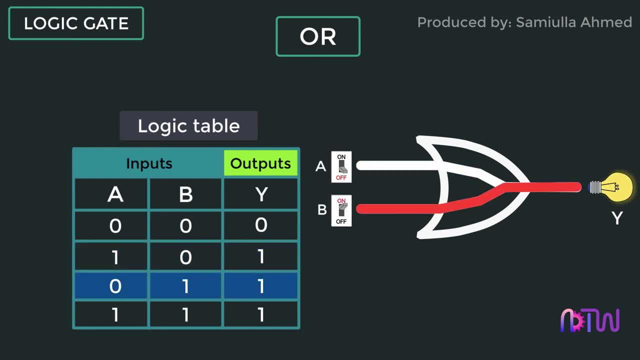 If switch B is on and switch A is off, still bulb will glow, And if both switches A and B are on, the bulb will glow. This is how OR gate works. If you are enjoying this video, please give this video a thumbs up, and if you are new to ADTW. 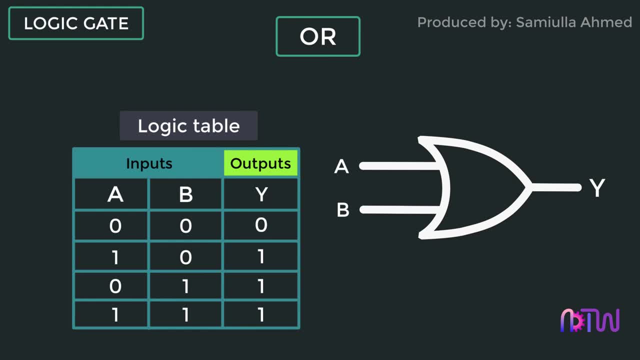 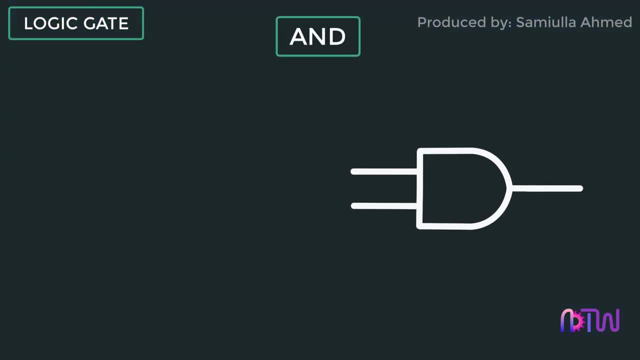 learn, click on the subscribe button and turn on the notification to get new information. Thank you for watching. Let's move on to next logic gate, which is AND gate. Similar to OR gate, AND gate also has two inputs, A and B, and one output, Y. The working of AND gate is based on the mathematical meaning of 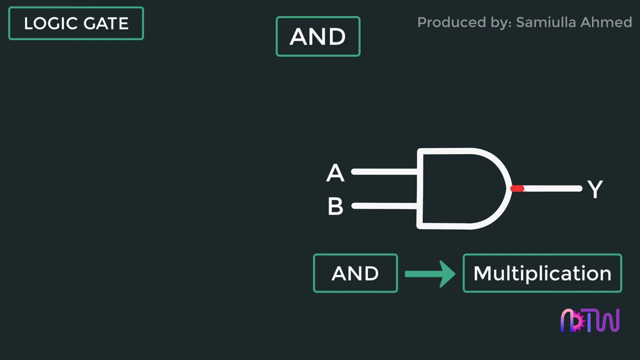 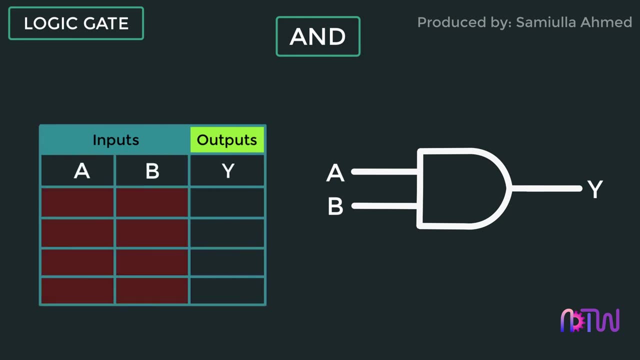 AND that is multiplication. For the AND gate to give an output, both the input, A and B, should have a signal. Let's see the logic table for AND gate. It can have four combinations of input. The first input will be A equals 0, and B equals 0. Since both A and B have no signal, the output Y will be 0.. You can also 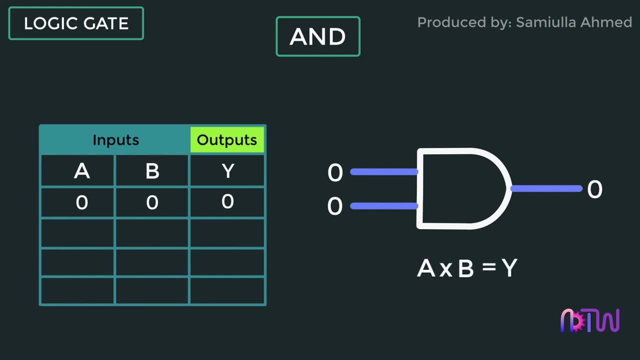 get the output of AND gate by doing A into B, Since A equals 0 and B equals 0, 0 into 0, will give the result equal to 0.. Second set of inputs will be A equals 1 and B equals 0.. Since only A, 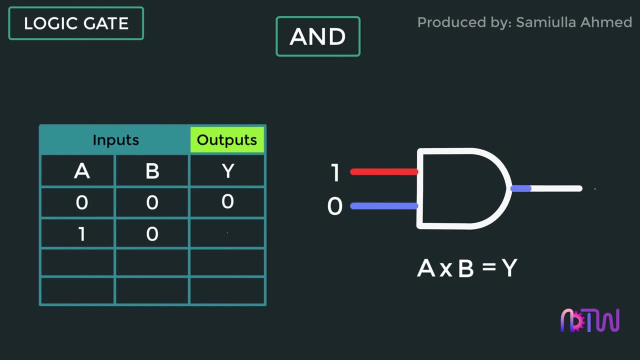 has an input and B doesn't, the output will be equal to 0.. Since A into B equals 0,, the output will be equal to 0.. Similarly, for the third input, A equals 0 and B equals 1, we will have the same. 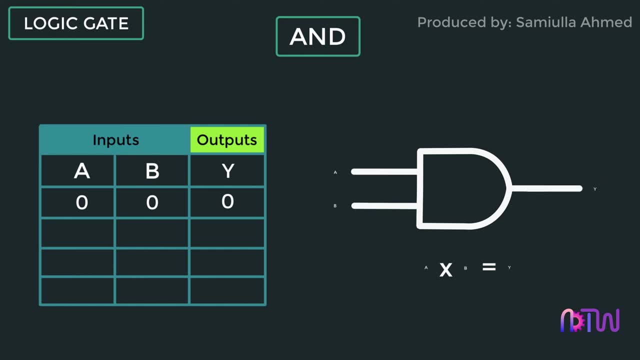 result equal to 0.. Second set of inputs will be: A equals 1 and B equals 0. Since only A has an input and B doesn't, the output will be equal to 0.. Since A into B equals Y, if we put A, 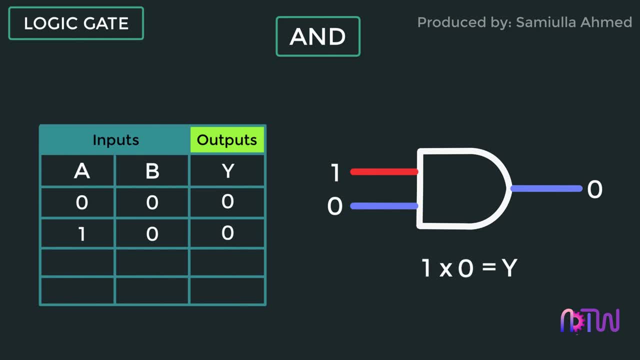 equals 1 into B equals 0, the output result from this operation will be equal to 0.. Similarly, for the third input, A equals 0 and B equals 1, we will have the same result. Since A equals 0 into B equals 1, results in output Y equals 0.. For the last set of inputs, which are: A equals 1. 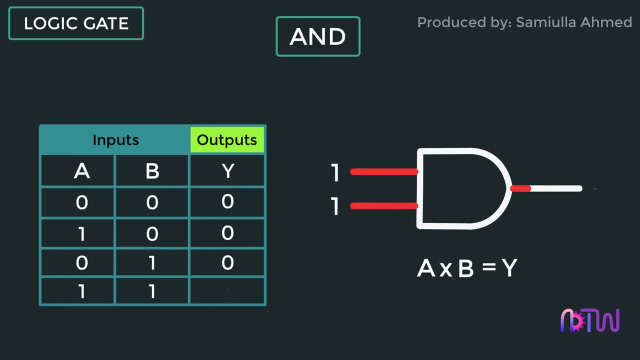 and B equals 1, we will have the output Y equals 1.. Since both A and B are having input 1, this will meet the condition to provide output 1.. We can even verify it by putting these inputs into equation: A into B equals Y. Since A equals 1 and B equals 1, 1 into 1 is equal. 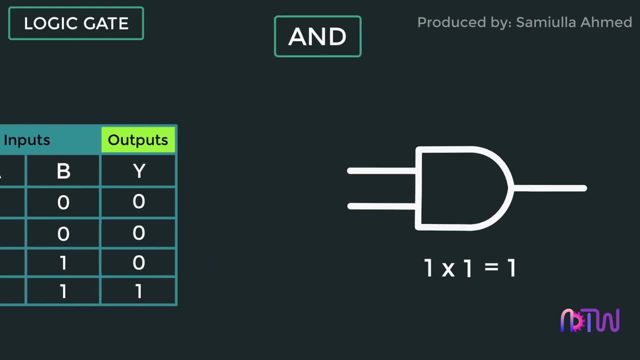 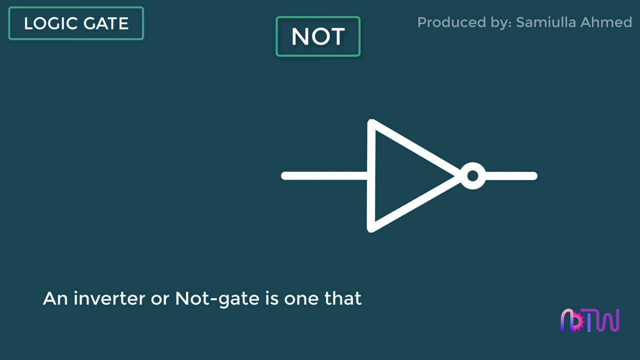 to 1.. This is the logic behind the working of AND gate. Next we will see how NOT gate works. An inverter or NOT gate is one that outputs the opposite state as what is input. It has only one input and one output. 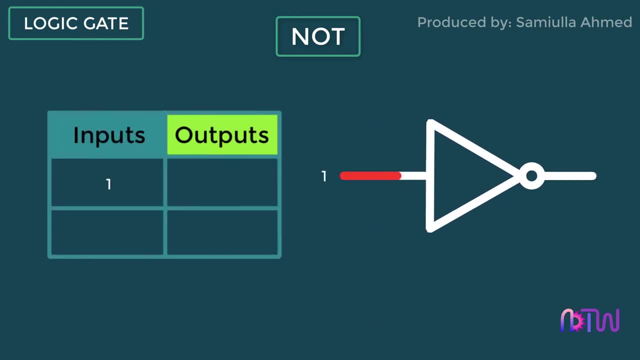 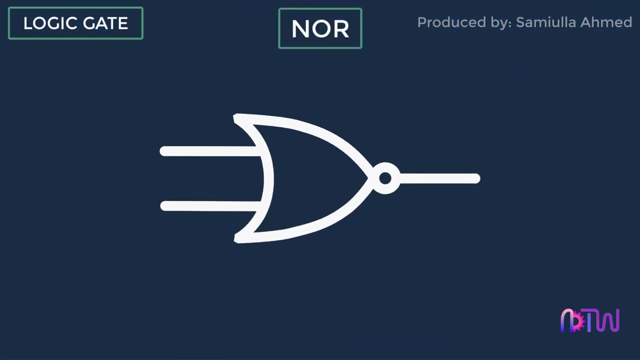 If you provide an input signal 1,, the output will be 0, and if you provide input signal 0,, the output will be 1.. This is how NOT gate works. Our next logic gate is NOR gate. NOR gate is the combination of OR gate and NOT gate. 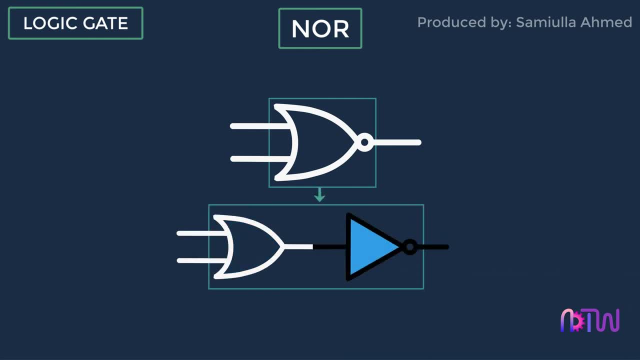 The output of the OR gate will pass through the NOT gate. Hence the output gets reversed. That is, if the output of OR gate is 1, then after passing through NOT gate, the output will be equal to 0. Therefore, NOR gate provides output opposite to the OR gate. 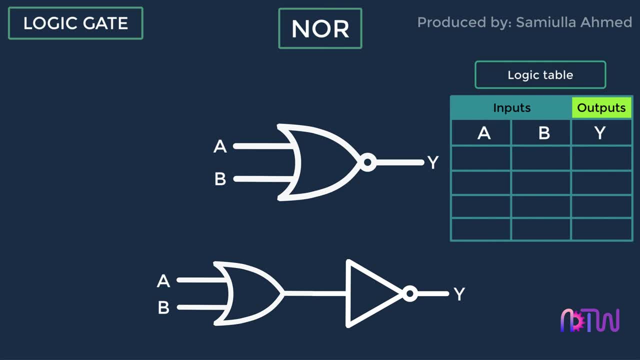 Let's see the logic table for NOR gate. For the understanding purpose, we will use the OR gate's logic table as a reference. Our first input will be: A equals 0 and B equals 0.. The OR gate output will be equal to 0.. 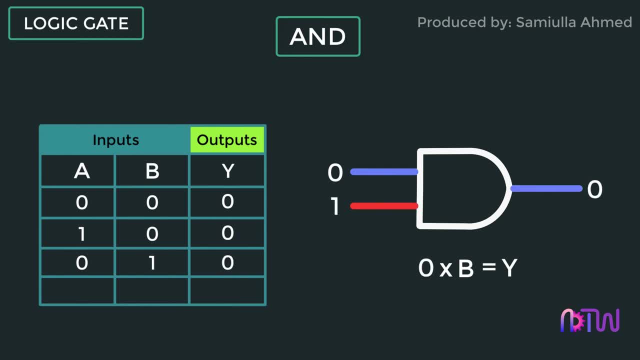 result: Since A equals 0 into B equals 1, results in output Y equals 0.. For the last set of inputs, which are A equals 1 and B equals 1, we will have the output Y equals 1.. Since both A and B 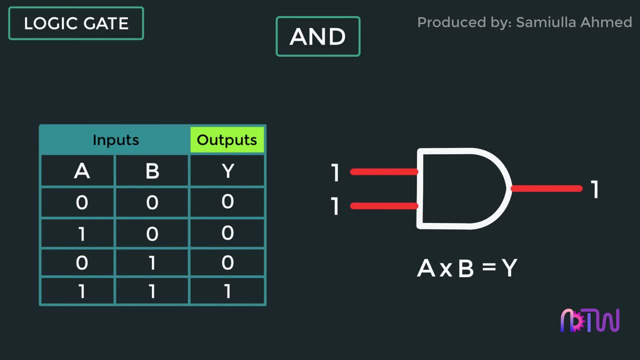 are having input 1,, this will meet the condition to provide output 1.. We can even verify it by putting these inputs into equation: A into B equals Y, Since A equals 1 and B equals 1.. 1 into 1, is equal to 1.. This is the logic behind the working of AND gate. 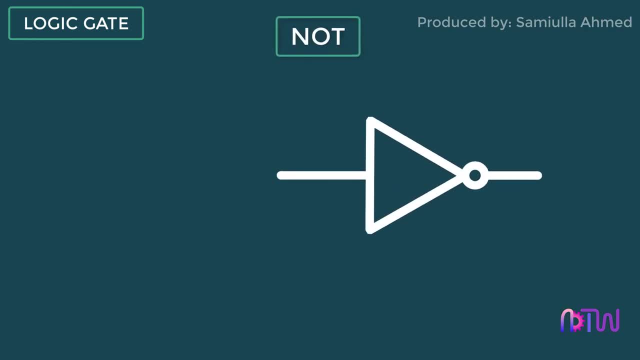 Next we will see how NOT gate works. An inverter or NOT gate is one that outputs the opposite state as what is input? It has only one input and 1 output. If you provide an input signal 1, the output will be 0. And if you provide input signal, 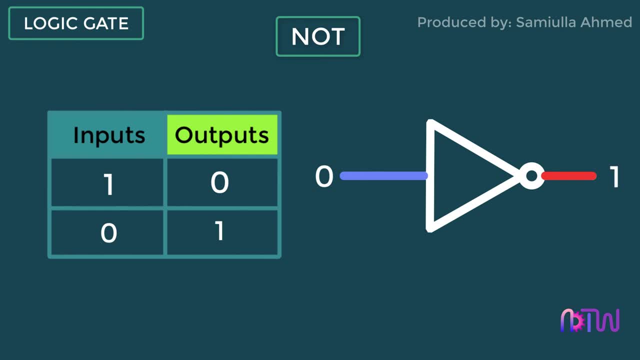 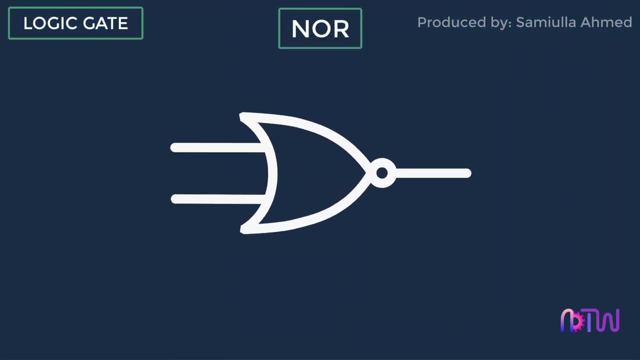 0,, the output will be 1.. This is how NOT gate works. Our next logic gate is NOR gate. NOR gate is the combination of OR gate and NOT gate. The output of the OR gate will pass through the NOT gate. Hence the output gets reversed. That is, if the output of OR gate is 1, then after passing 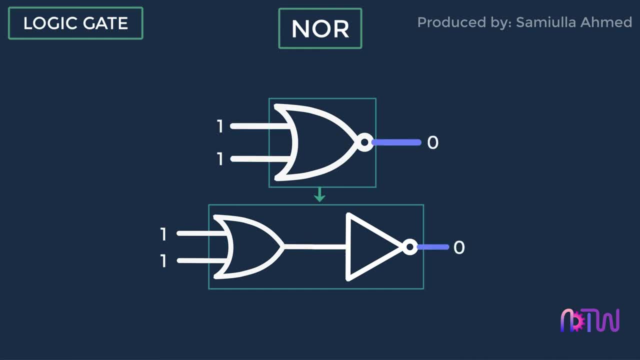 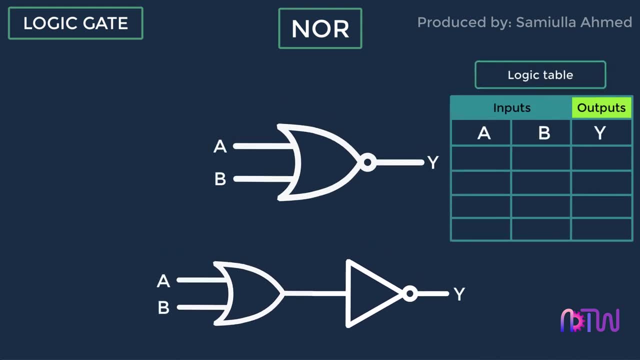 through, NOT gate, the output will be equal to 0. Therefore, NOR gate provides output opposite to the OR gate. Let's see the logic table for NOR gate. For the understanding purpose, we will use the OR gate's logic table as a reference. Our first input will be: A equals 0 and B equals 0.. The OR 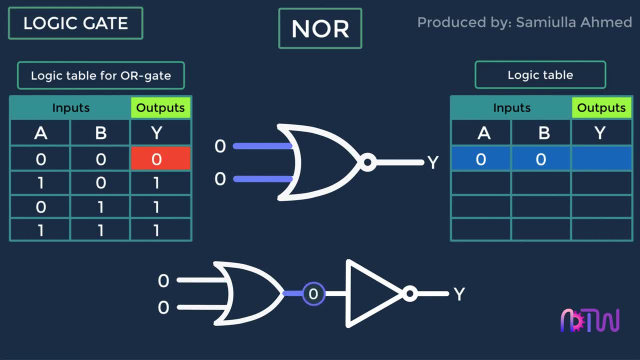 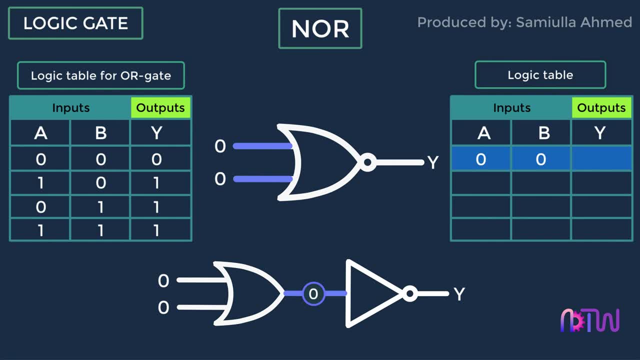 then pass through NOT gate, which reverses the input 0 into the final output 1.. Second set of inputs will be A equals 1 and B equals 0. The output after passing through OR gate will be equal to 1.. Then again, passing this input through the NOT gate, we will have a final output as 0.. 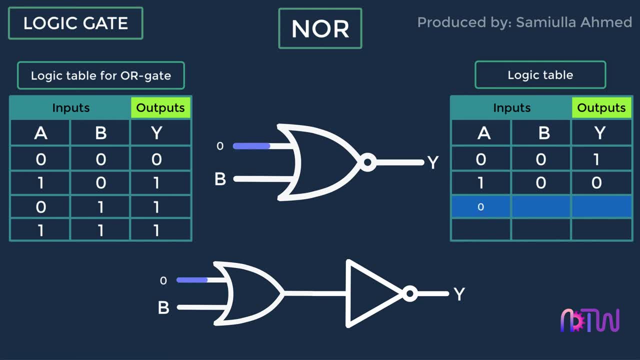 The next set of inputs will be A equals 1 and B equals 0.. The output after passing through OR gate will be A equals 1 and B equals 0.. The next set of inputs will be A equals 0 and B equals 1.. The 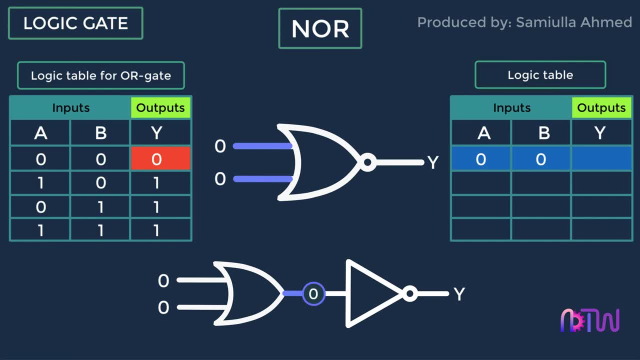 But, as we can see, we have NOT gate after the OR gate. The output 0 will then pass through, NOT gate, which reverses the input 0 into the final output 1.. Second set of inputs will be A equals 1 and B equals 0.. 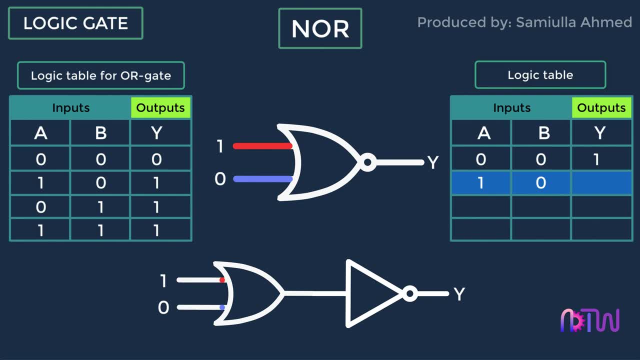 The output after passing through OR gate will be equal to 1.. Then again, passing this input through the NOT gate, we will have a final output as 0.. The next set of inputs will be A equals 0 and B equals 0.. The output of OR gate with these input signals will be equal to 1.. 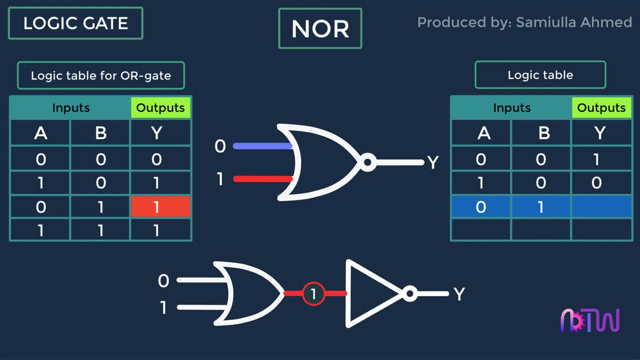 After passing the output of OR gate through the NOT gate, we will have the final output as 0.. Since NOT gate reverses whatever input it gates And the final set of input signals will be A equals 1 and B equals 1.. 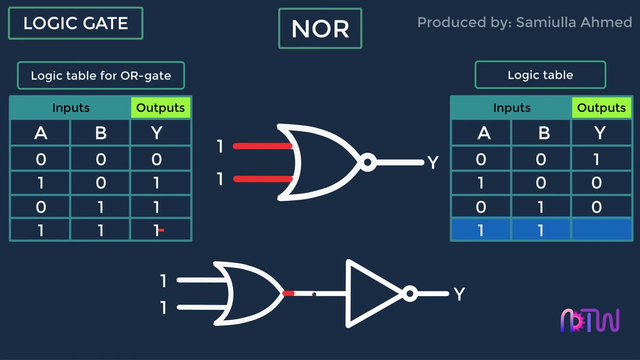 For these input signals, the output of the OR gate will be 1.. After passing through the NOT gate, the final output will be 0.. In short, we can say that the output of the NOR gate is opposite to the output of the OR gate. 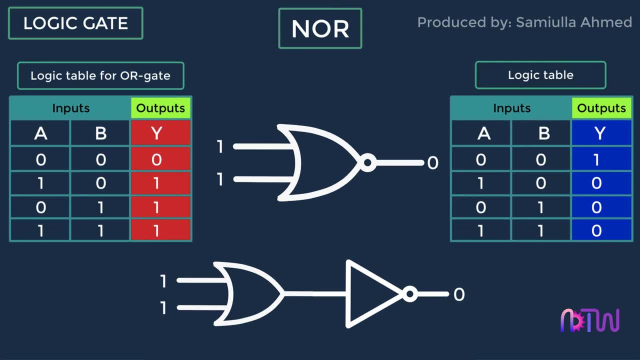 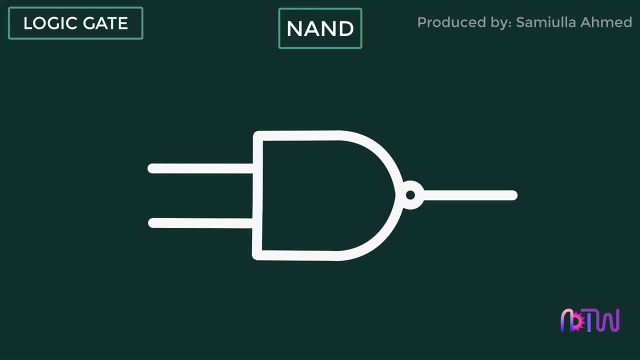 This is how NOR gate works. Let's move on to our next gate, which is NAND gate. As we saw how OR gate's output is passed through the NOT gate to get the opposite results of OR gate. Likewise, the AND gate's output is passed through the NOT gate to get opposite results of AND gate for the same set of inputs. 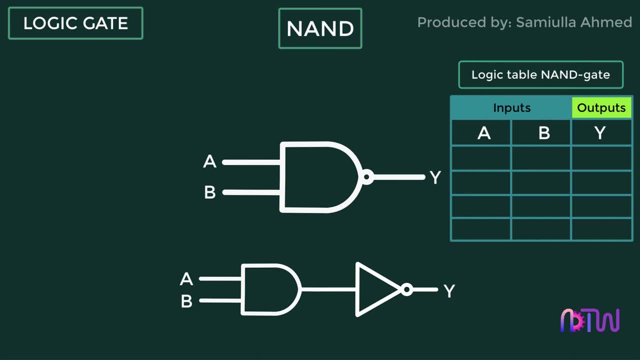 Let's see the logic table for NAND gate. For understanding purposes we will keep the AND gate's logic table for reference. The first inputs will be A equals 0 and B equals 0.. The output of AND gate will be 0.. 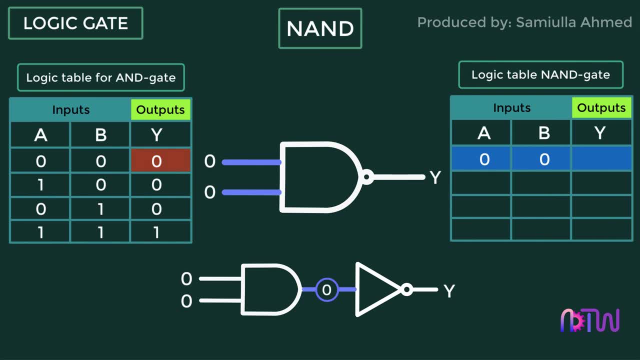 After passing this output through the NOT gate, we will have the final output as 1.. For second set of inputs, A equals 1 and B equals 0. The output of AND gate for these inputs will be 0.. After passing through the NOT gate, we will have the final output as 1.. 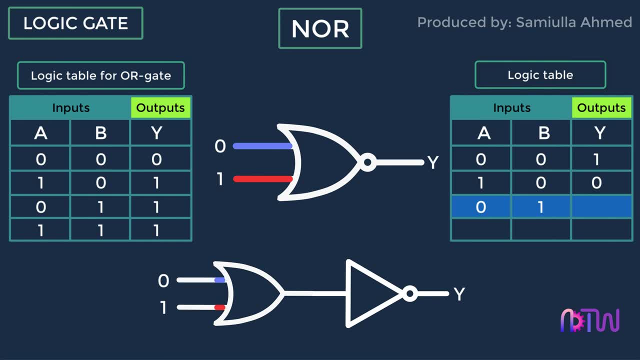 output of OR gate with these input signals will be equal to 1.. After passing the output of OR gate through the NOT gate, we will have the final output as 0.. Since NOT gate reverses whatever input it gates And the final set of input signals will be A equals 1 and B equals 1.. 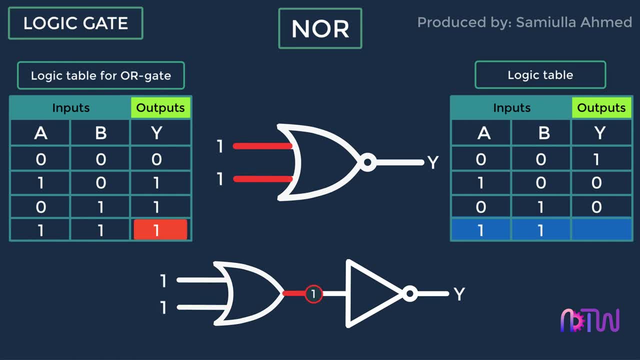 For these input signals, the output of the OR gate will be 1.. After passing through the NOT gate. to this result, the output from OR gate is equal to 1.. Because we have라고 a number of rooms, we experimented with the solution and we saw that the output from the 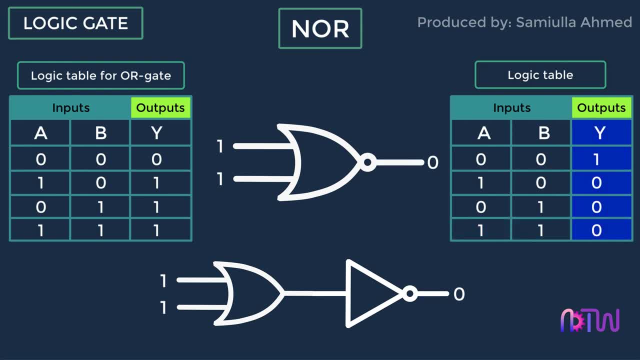 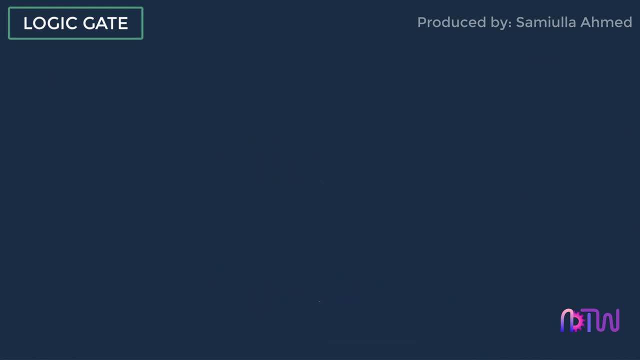 OR gate would be 0.. When we have due to the Это to通 and con result ≒ the OR gate, the final output will be 0.. In short, we can say that the output of the NOR gate is opposite to the output of the OR gate. This is how NOR gate works. 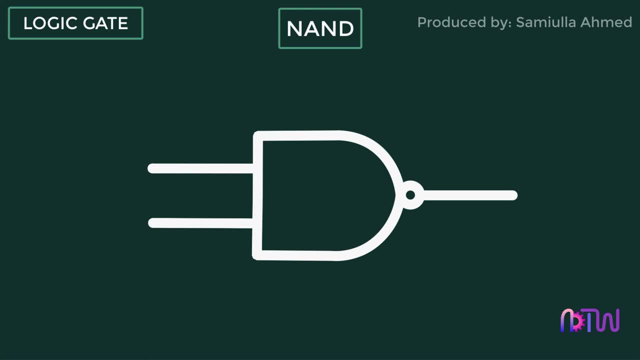 Let's move onto our next gate, Which is an AND gate. As we saw how OR gate's output is passed through the NOT gate to get the opposite results of OR gate. Likewise, the AND gate's output is passed through the not gate to get opposite results of AND gate for the same reason, versus. 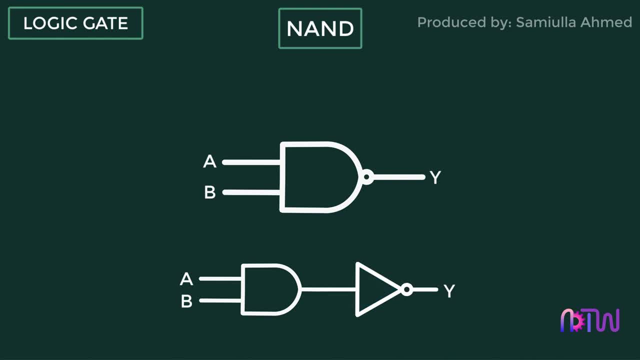 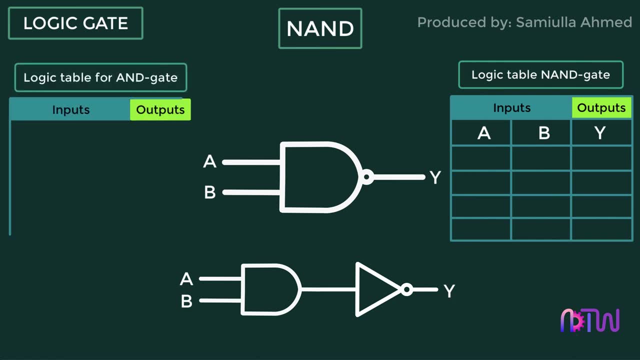 the AND gate. in any case, If we elements this output into the AND gate, then it delivers results of AND gate for the same set of inputs. Let's see the logic table for NAND gate For understanding purposes. we will keep the AND gate's logic table for reference. 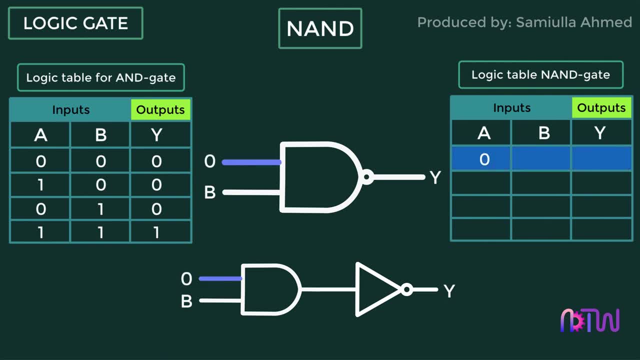 The first inputs will be A equals 0 and B equals 0.. The output of AND gate will be 0.. After passing this output through the NOT gate, we will have the final output as 1.. For second set of inputs: A equals 1 and B equals 0.. The output of AND gate for these: 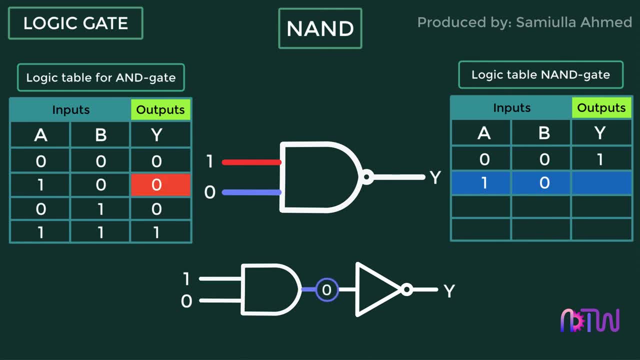 inputs will be equal to 0.. After passing through the NOT gate, we will have the final output as 1.. Similarly, for third set of inputs, A equals 0 and B equals 1.. The output of AND gate for these inputs will be 0.. After passing through 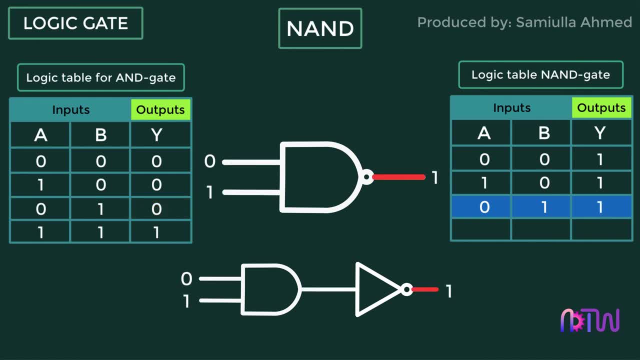 the NOT gate, we will have the final output as 1.. For the last set of inputs, A equals 1 and B equals 0.. The output of AND gate for these inputs will be 0.. After passing through the NOT gate, we will have the final output as 1.. 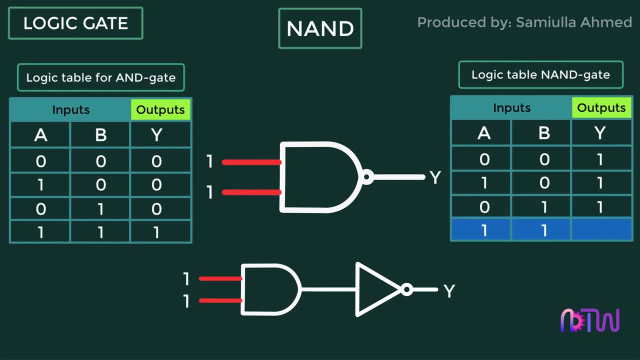 inputs A equals 1 and B equals 1.. The AND gate's output will be 1.. But after passing this input through the NOT gate, we will have the final output as 0. Therefore, we can see that the output of the NAND gate is opposite to the output given by the AND gate. 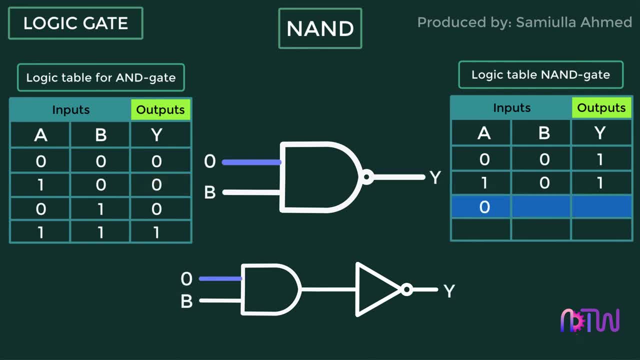 Similarly, for third set of inputs: A equals 0 and B equals 1.. The output of AND gate for these inputs will be 0.. After passing through the NOT gate, we will have the final output as 1.. For the last set of inputs: A equals 1 and B equals 1.. 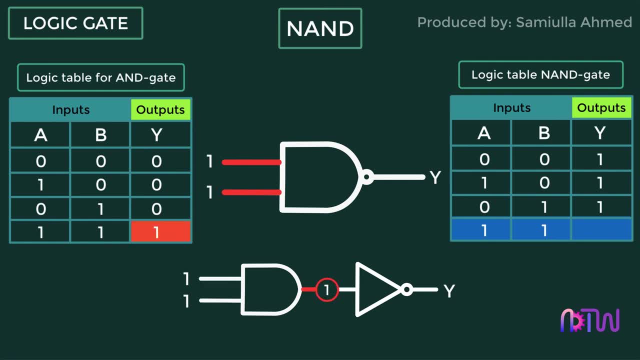 The AND gate's output will be 1.. After passing this input through the NOT gate, we will have the final output as 0. Therefore, we can see that the output of the NAND gate is opposite to the output given by the AND gate. 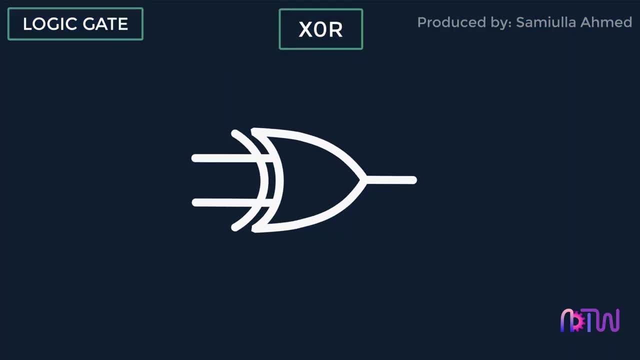 Next we will see exclusive OR gate. The specialty of exclusive OR gate is that it gives an output when there is a signal in only one of the inputs. It will not provide any output signal if both the inputs are 0 or both the inputs are 1.. 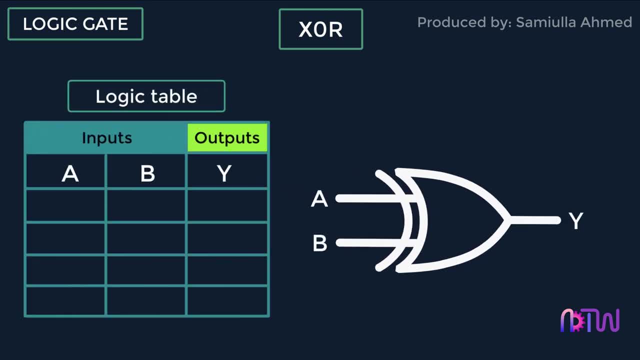 Let's see the truth. table for exclusive OR gate. Since it has two inputs, there can be four combinations of inputs. For first set of inputs, A equals 0 and B equals 0.. The output of exclusive OR gate will be 0.. 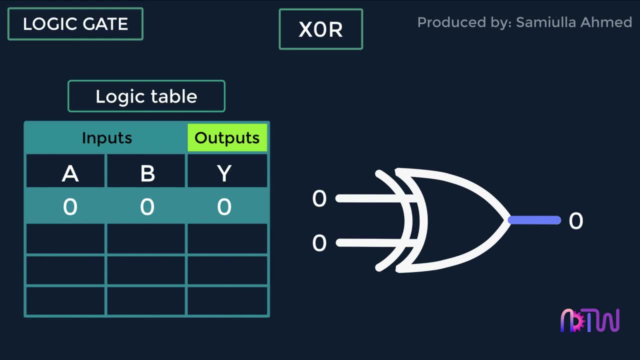 Since there is no signal in both the inputs, Second set of inputs will be A equals 1 and B equals 0. Since there is a signal in one of the inputs, therefore, the output will be 1.. Similarly, if A equals 0 and B equals 1.. 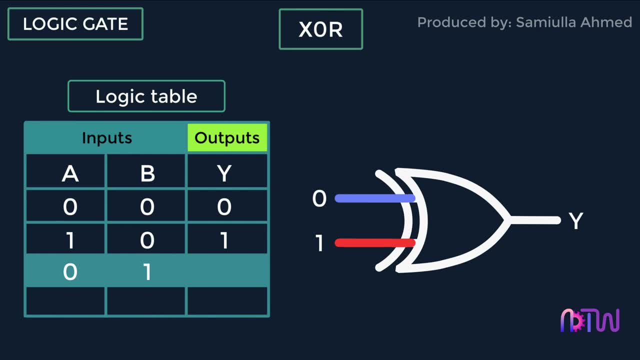 Still, the output signal from this logic gate will be 1.. And the final set of inputs, A equals 1 and B equals 1.. In this case, the output signal will be 0. Because for exclusive OR gate to work, only any one of the signals should be high. 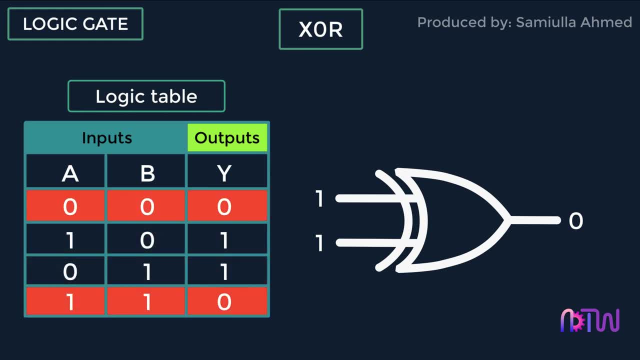 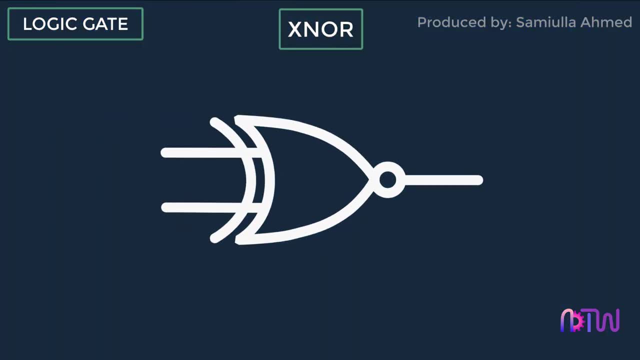 If both signals are high or low, then the output signal will be 0.. Next, and the final logic gate is exclusive NOR gate, As we have seen how NOR gate and AND gate have been created to get a complement output of OR gate and AND gate. 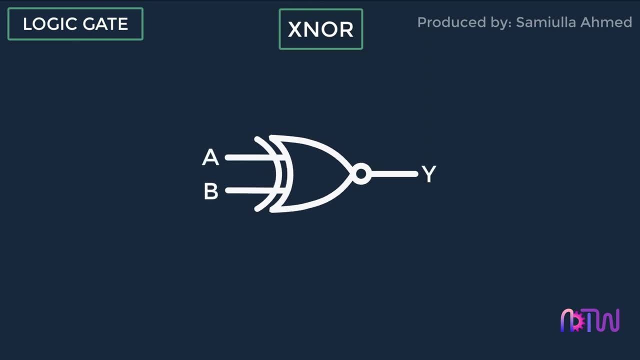 Similarly, the exclusive NOR gate is developed by combining exclusive OR gate with NOT gate. The output signal of the exclusive OR gate is passed through the NOT gate to get a complement output of the exclusive OR gate. Let's see the logic table for exclusive NOR gate. 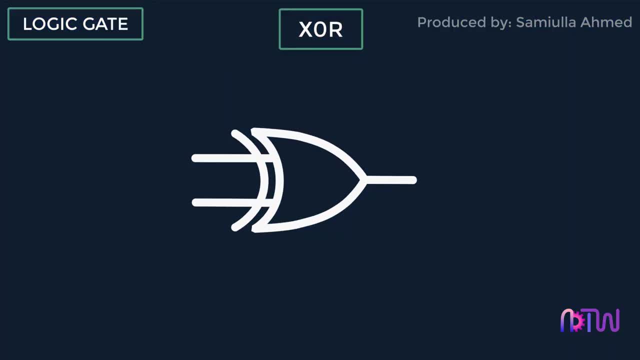 Next we will see exclusive OR gate. The specialty of exclusive OR gate is that it gives an output when there is a signal in only one of the inputs. It will not provide any output signal if both the inputs are 0 or both the inputs are 1.. 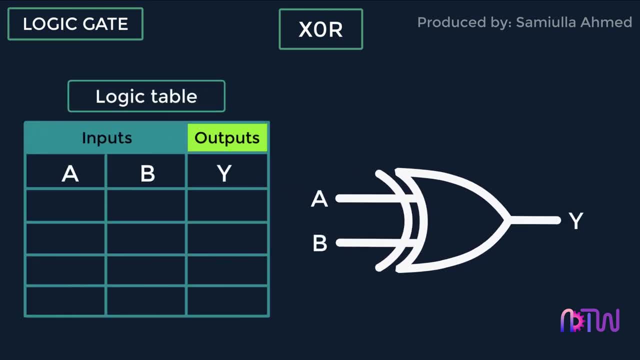 Let's see the truth table for exclusive OR gate. Since it has two inputs, there can be four combinations of inputs. For first set of inputs, A equals 0 and B equals 0. The output of exclusive OR gate will be 0. Since there is no signal in both the inputs. 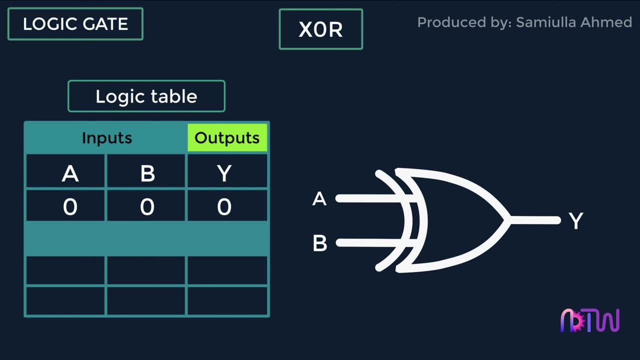 Second set of inputs will be A equals 1 and B equals 0. Since there is a signal in one of the inputs, therefore the output will be 1.. Similarly, if A equals 0 and B equals 1. Still, the output signal from this logic gate. 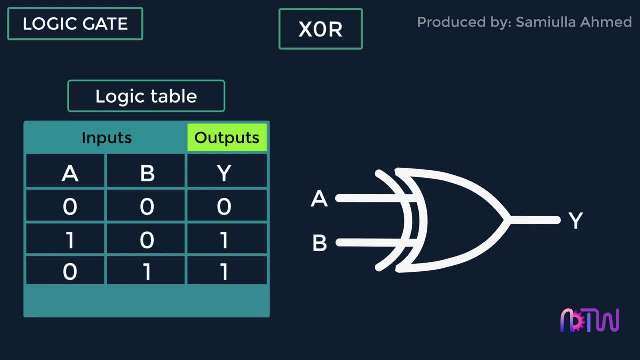 will be 1.. And the final set of inputs, A equals 1 and B equals 1.. In this case, the output signal will be 0.. As for exclusive OR gate, to work only any one of the signals should be high. If both. 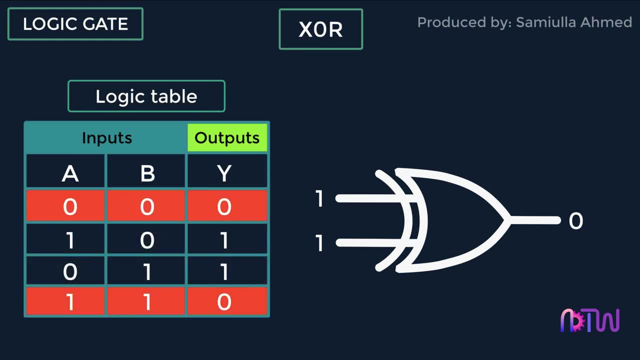 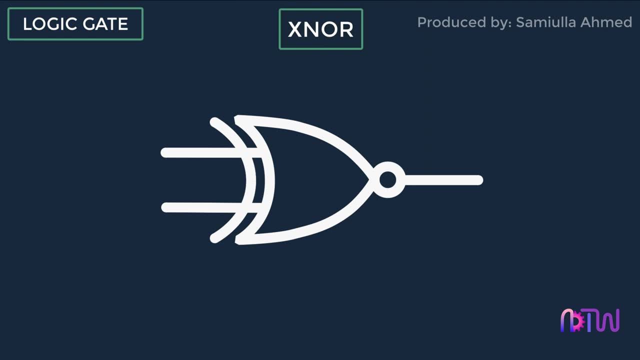 signals are high or low, then the output signal will be 0.. Next, and the final logic gate is exclusive NOR gate, As we have seen how NOR gate and AND gate have been created to get a complement output of OR gate and AND gate. Similarly, 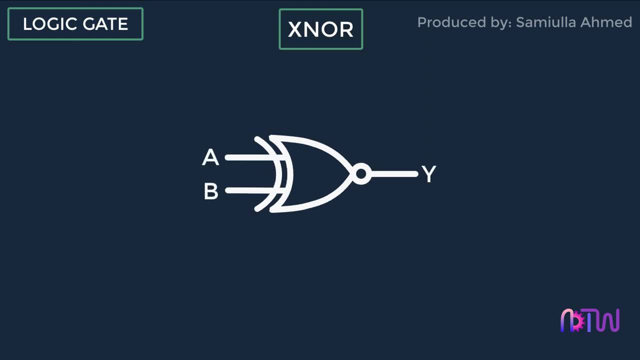 the exclusive NOR gate is developed by combining exclusive OR gate with NOT gate. The output signal of the exclusive OR gate is 0.. The output signal of the exclusive OR gate is 0.. The output signal is passed through the NOT gate to get a complement output of the exclusive. 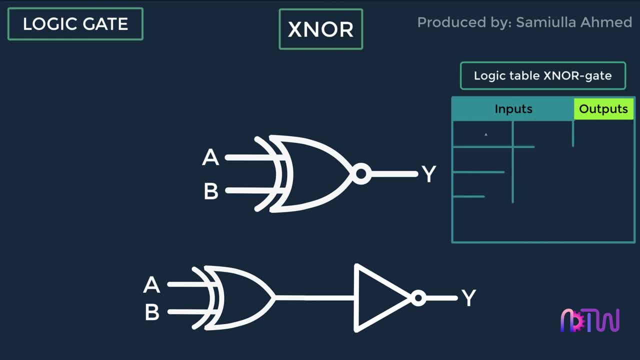 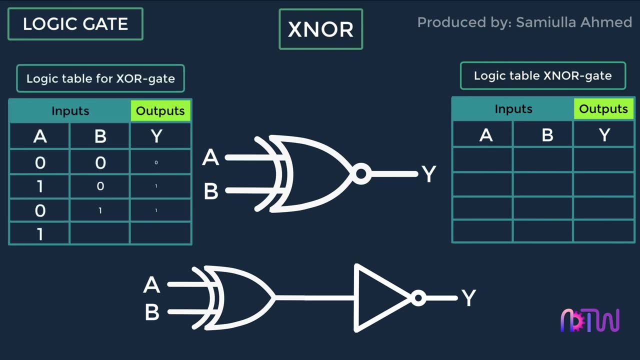 OR gate. Let's see the logic table for exclusive NOR gate. For the understanding purpose, we will keep the logic table of exclusive OR gate for reference. Now our first set of inputs will be: A equals 0 and B equals 0.. The output from the exclusive. 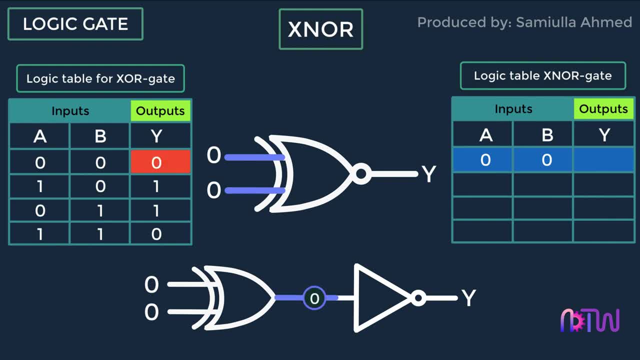 OR gate will be equal to 0,, but after passing through the NOT gate, The final output signal will be 1.. The second set of inputs will be A equals 1 and B equals 0.. The output from the exclusive OR gate will be 1,, but after passing through the NOT gate, The final output signal will